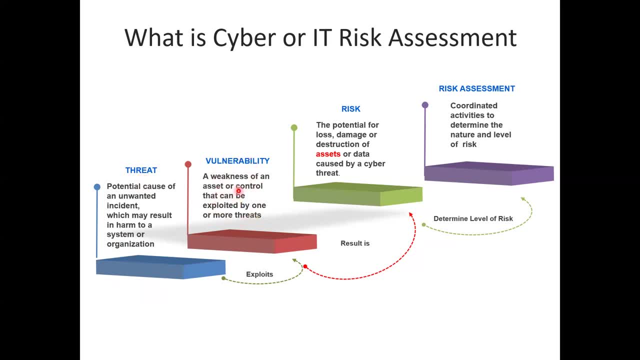 So that means in your system or your network or your asset is a loophole, It's a weakness that the threat actors can take advantage of, And when this happens, the result is what you see as risk. So it means that. so risk occurs when threat exploits vulnerabilities. 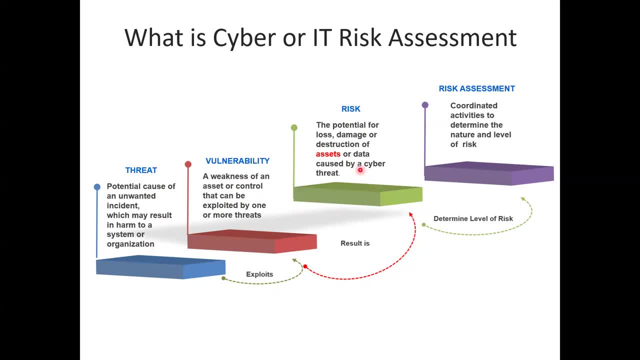 And the result, like I said, is risk. So what is the risk? in itself, Risk is potential for loss, damage or destruction of asset or data, you know, which can be caused by cyber threat. You know so, when there is a weakness in the system, or vulnerability, as we say, the threat actors also looking out for vulnerabilities in the system. 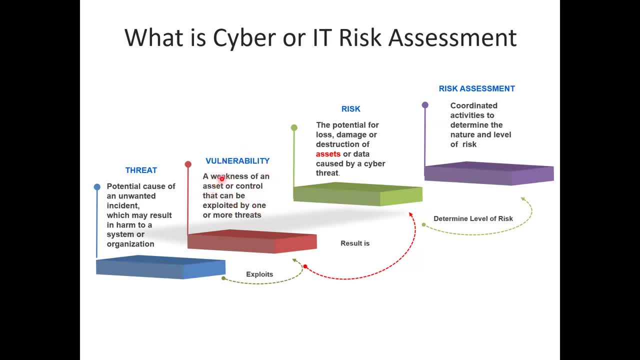 And then, when they see a vulnerability, they take advantage of it and they exploit it And, what you see, they can expand to harm your system, your harm, your network or your data, your laptop, your server, whatever the asset is. 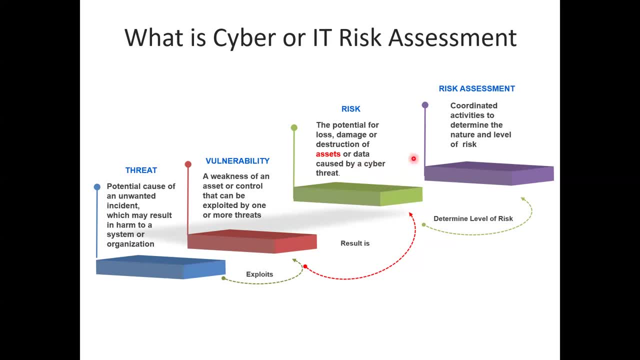 And so now, what, then, is risk assessment? You know, remember, that when a risk happens, we need to be able to find out or determine what is the level of the risk. Some risk out, Some risk out Minimal, Some are high. 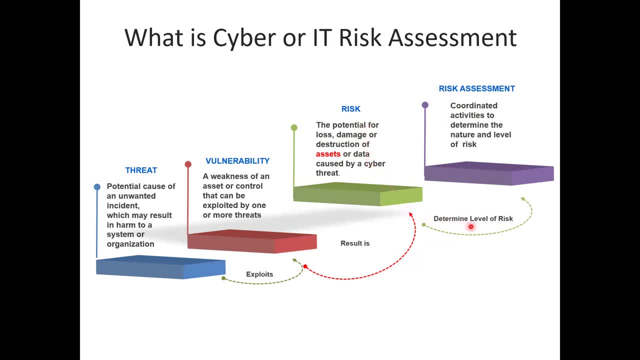 Some are low, Some are medium, You know. so the process of determining the level of the risk that has happened is what is known as risk assessment. So it's a coordinated activity to determine the nature and the level of risk, Because every risk, like I said, has level. 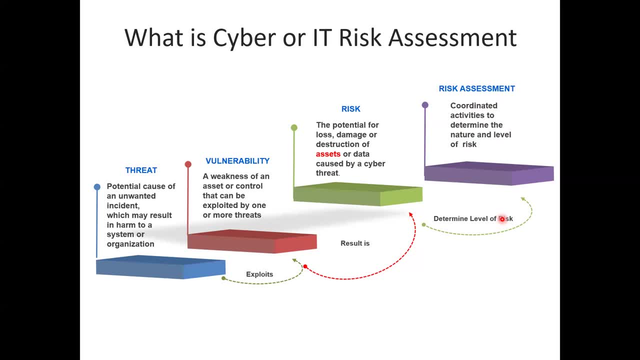 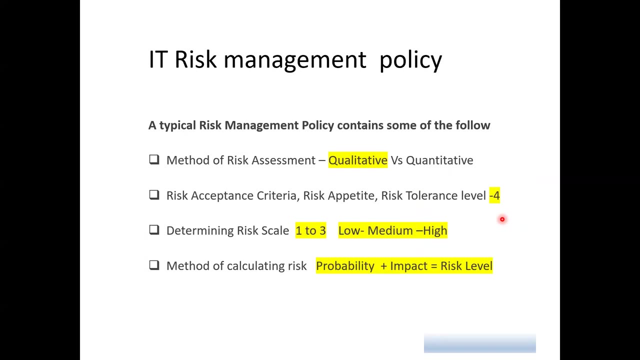 It could be low risk, It could be high risk, You know. so that is just a brief introduction of some of the terminology, Of some of the terminologies relating to risk assessment. And so, ideally, in the real world, in an organization, in a company, before you talk about risk assessment, the organization should have what is called IT risk management policy or risk management policy. 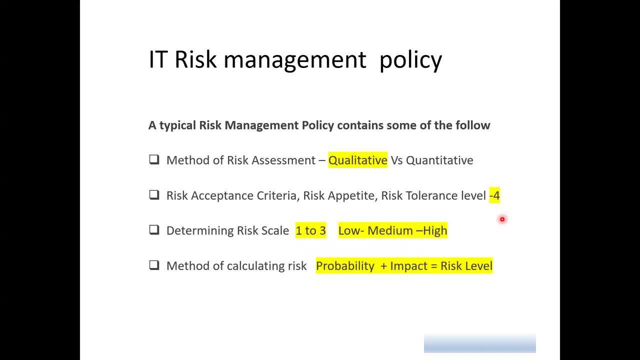 So the policy contains information on how the company wants to manage their IT risk, How they want to conduct risk assessment, Information on how they want to conduct risk treatment, Information on how to identify risk and everything about risk management is contained in that document. 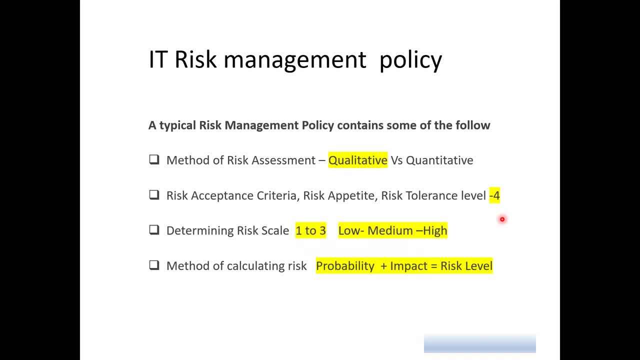 But for the purpose of this video, I've only extracted a section of the risk policy of a particular organization And that has to do with risk assessment. So, like I said before, organizations usually would document how they want to conduct risk assessment. Remember, we are dealing with risk assessment. 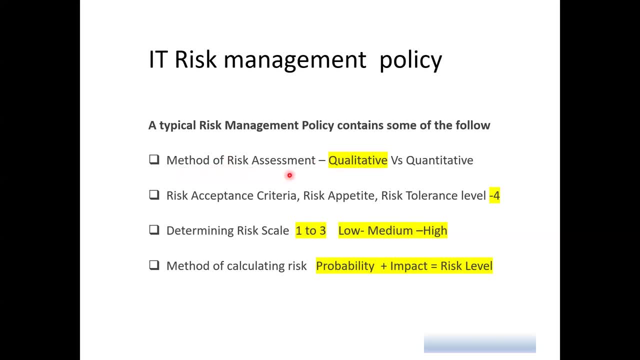 So they document the method they want to use in conducting risk, whether qualitative or quantitative. Qualitative means they are going to be using, like risk scales, scale of figures of 1, 2, 3, 1, 2, 3, 4, 5- to determine their risk level. 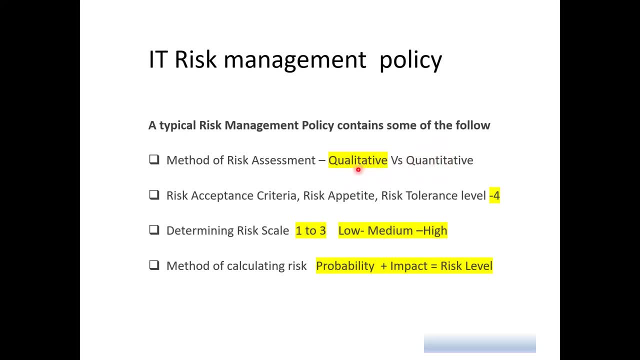 Quantitative is that instead of using 1,, 2,, 3,, 4, 5 or risk scale, you use absolute figures Instead of saying: my risk level is 5.. Quantitative would say: no risk level is about $2,500 or £2,500. 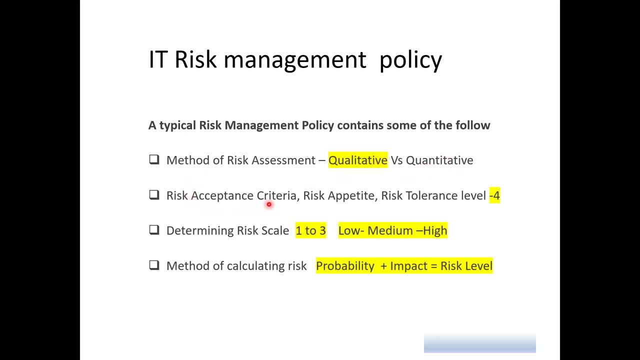 So that is the difference. And so in the policy also the company would document what is their risk acceptance criteria, or what you call as risk appetite, or what you call risk tolerance level. In other words, they would say in their risk policy: any risk that we assess. 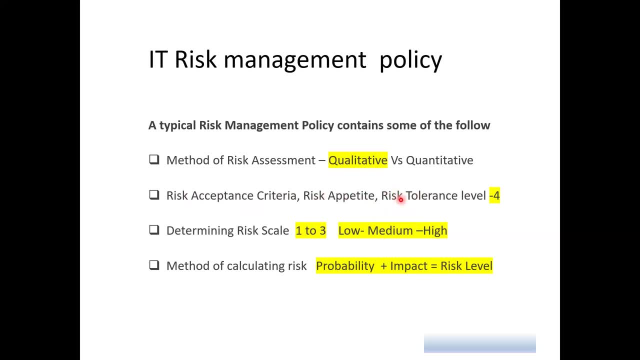 And the risk is above a particular level, We would have to do something about the risk. We have to treat that risk or reduce that risk or mitigate that risk. Yeah, So if, after determining their risk level, and they find out that their risk level is above that minimum or maximum tolerance limit, then that risk has to be treated. 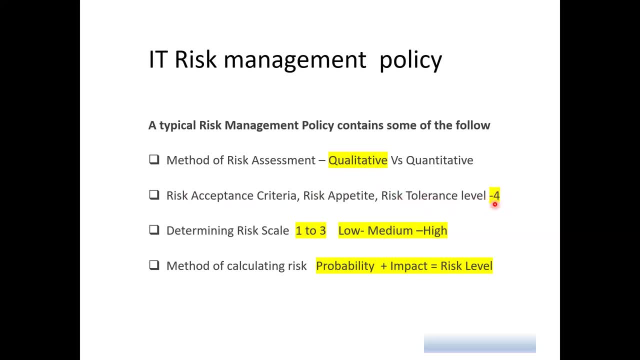 So, for example, we have taken, for the purpose of this video, We have used risk level 4 as the risk tolerance level for this video. We also use the qualitative method of assessing risk for this video. So what it means? that any risk that we calculate and it's above level 4, that means it has to be treated. 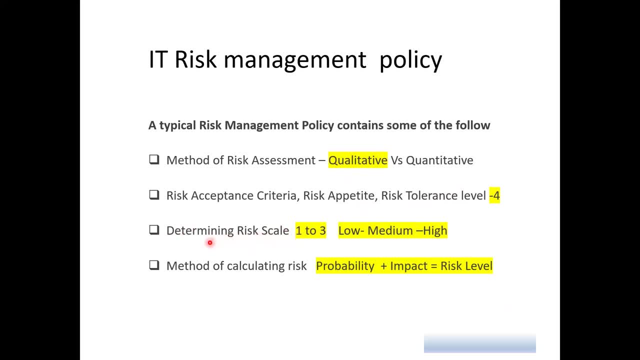 And so in the policy also, the company will also determine what their risk scale would be. Some people use a scale of 1 to 3.. So the low, medium, high, Where low, Where 1 is a low risk, Yeah. 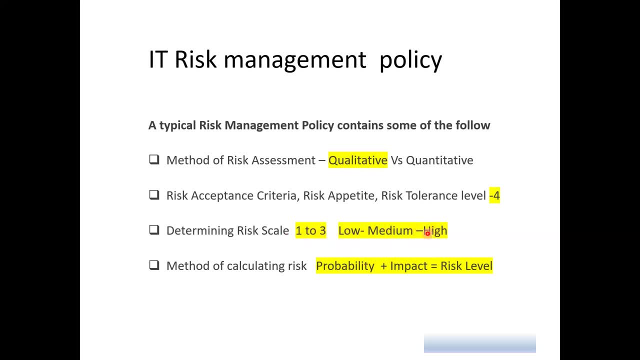 2 is a high risk. 2 is a medium risk, 3 is a high risk. Some of us organizations can use a scale of 1 to 5. That means it's going to be very low, low, medium, high and very high. 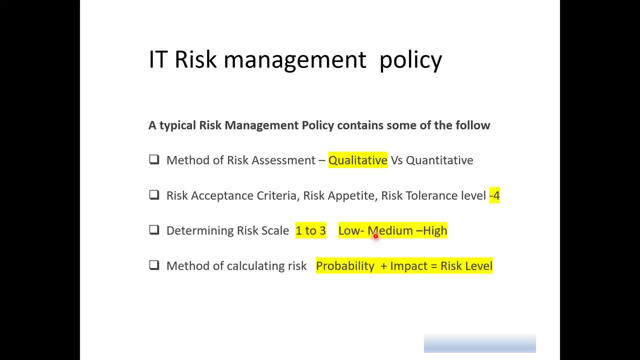 But for the purpose of this video our risk scale is going to be 1 to 3.. And then method of calculating risk. Organizations also document in their policy how they want to calculate their risk level. So ideally, risk level is a function of probability. 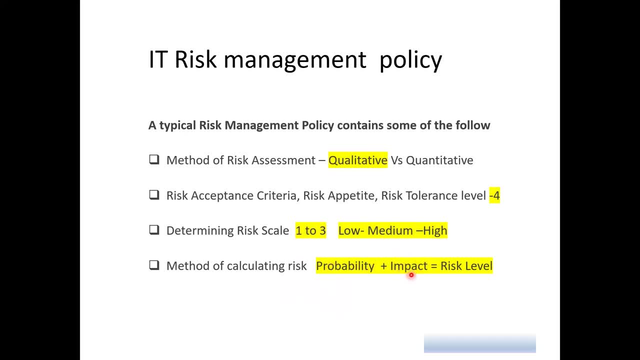 Probability and impact. So it's either you add both of them or you multiply both of them. So what organization determine? dependent on what the organization want to do. So for this purpose we want to use addition. Probability plus impact give us our risk level. 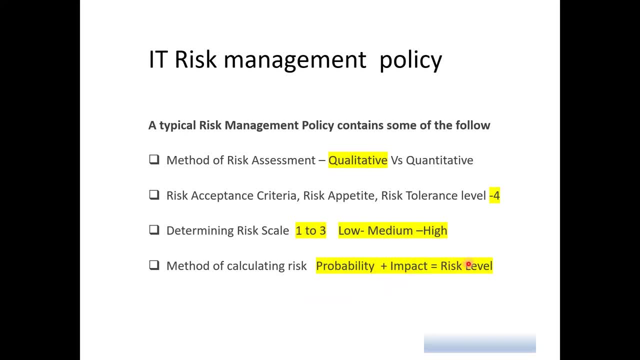 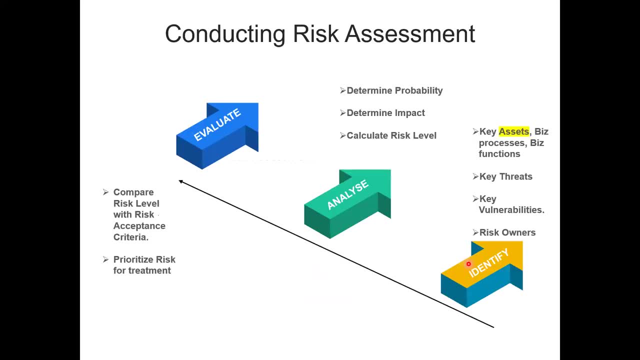 So this is a typical section of the company policy. Remember I said that the best thing for organization to do is to have a risk management policy. So let us go to the main business of the day, which is talking about risk assessment. We've defined risk. 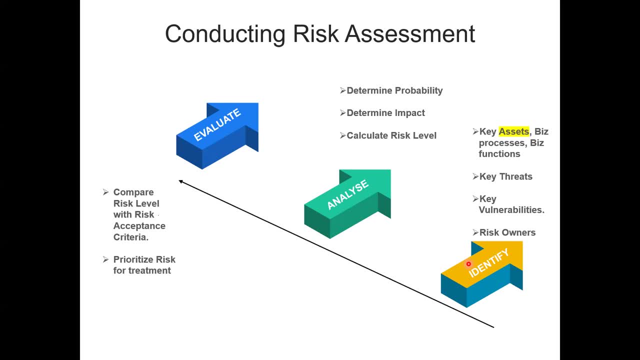 We've defined the key variables. So, in the process of risk assessment, what is the first thing you need to do? The first thing you need to do, by going from right to left, is to identify some key risk variables or key risk elements. And what are these elements which I've defined before? 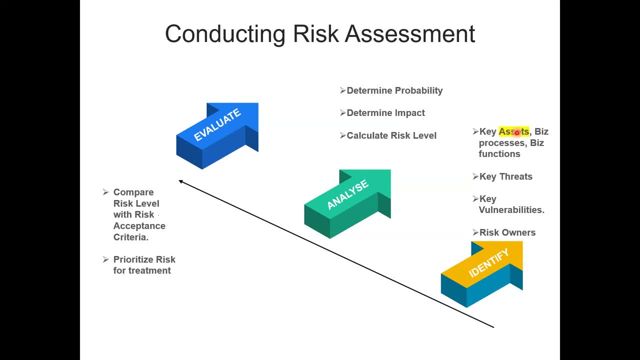 Identify the key risk elements. Identify the key risk elements. What are the key assets of the organization? What are the key IT assets of the organization? Assets could be server, your software, your application, router, network, And then also, apart from identifying the asset, you need to also identify the key threats that this asset can be exposed to. 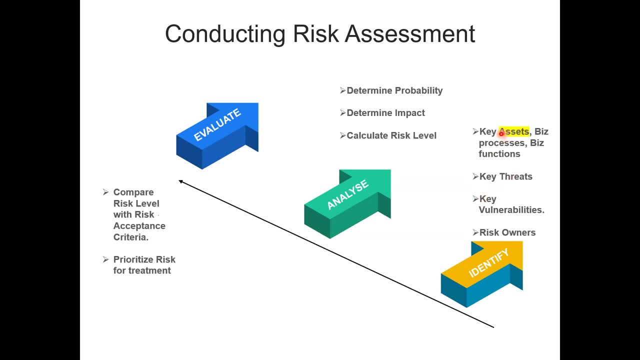 What can go wrong with this asset? What are the threats that they are facing? Also, we also identify the key vulnerabilities. What are the vulnerabilities that the assets have? What are the loopholes, What are the weaknesses on the assets that the threat actors can exploit? 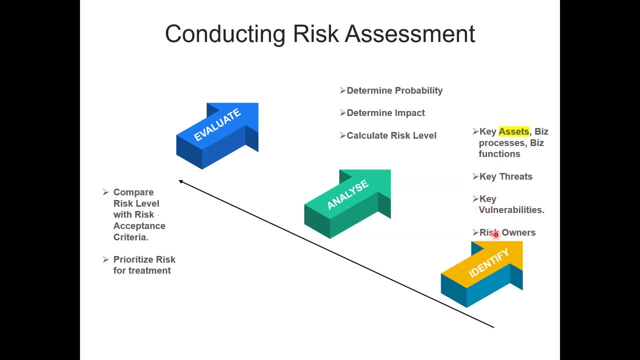 And then also the next thing we identify is identify the risk owners. Who are the risk owners? The risk owner is anybody that is responsible for managing a particular risk. Who are the risk owners? The risk owner is anybody that is responsible for managing a particular risk. 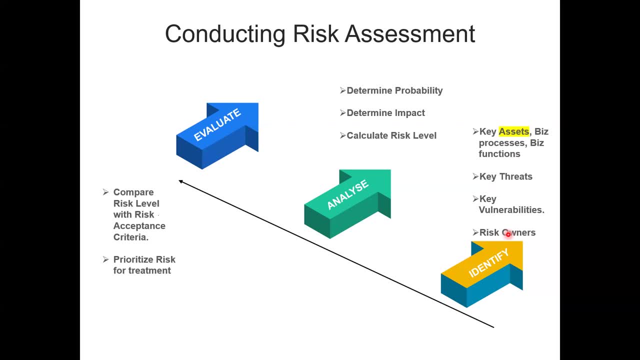 So in your risk assessment, you identify the three things we mentioned above here, But you also identify who the risk owner is. It should be a human, For example. it's like if you are assessing an asset or a business or a function or a department, assessing their risk. 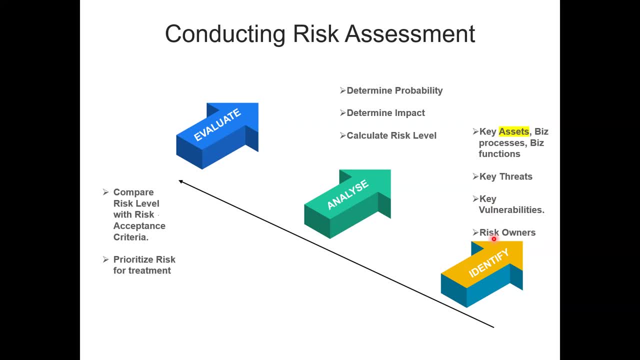 Maybe, for example, you are assessing the risk that has to do with HRD. Maybe, for example, you are assessing the risk that has to do with HR department. It means that the risk owner has to be the HR manager, because it's the one that we will be able to address or mitigate or do something about those risks that are identified. 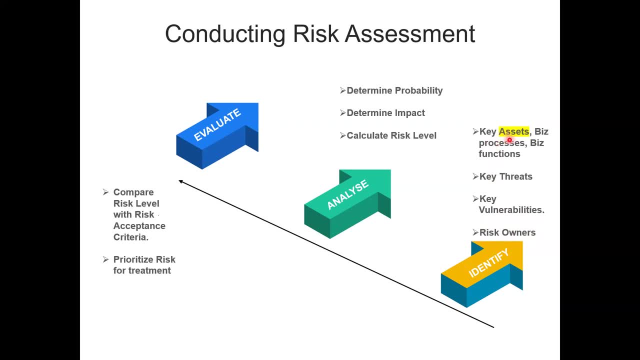 So that is a risk owner. So don't forget also that risk assessment is not only on IT asset. You can conduct risk assessment on business process, business procedure. You can conduct risk assessment on business function or a business department, for example on mining. 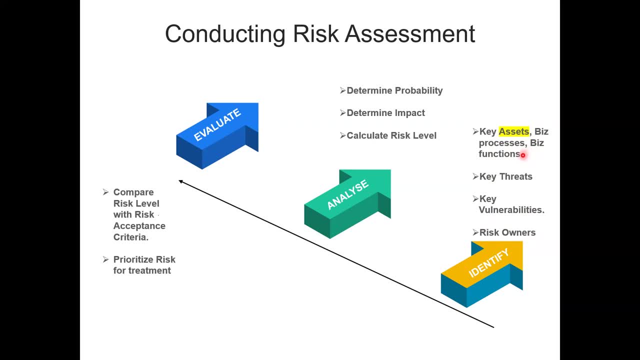 For example, you can conduct risk assessment on human resources procedure, the hiring procedure or the termination procedure. You can conduct the risk associated with that. So risk assessment is both on asset and also on processes, and also on functions as well, and also on department. 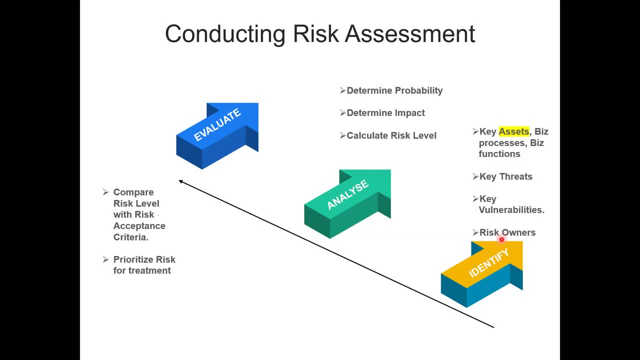 So, having identified this, the next thing is to now determine what is the probability. You know, we have analyzed here, we have evaluated here, but sometimes it can be confusing. But once you identify these key variables, the next thing is to now determine what is the probability of the risk happening. 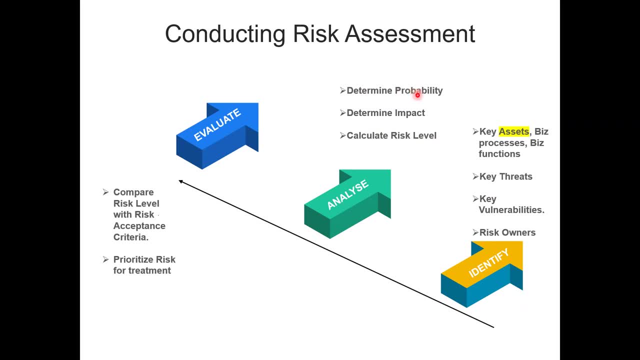 So you are determining the probability level And then what is the probability of the risk happening? You know you can say okay, is it possible it's going to happen, Why will it happen? Why will it not happen? And then if the probability is not very high, you can give it a low probability, like, okay, I can say okay. 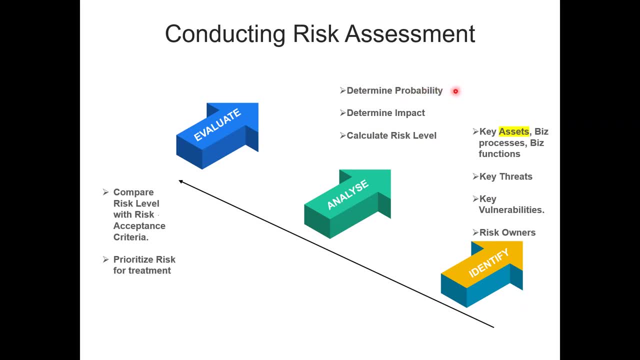 let's see what happens. Now, the probability is not too much, it can be one. And then I also could determine the impact level. the impact level, what will be the impact level if it happens? Okay, the impact. the probability is low, but the impact can be high if it happens. 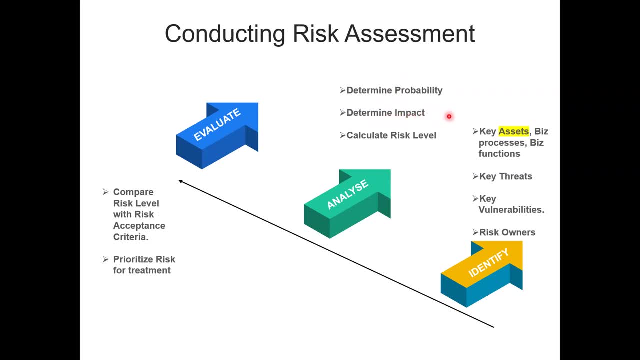 And so I can say, okay, the impact level is maybe three. Yeah, that is high, if it happens. So in that case, we have one as the probability level, we have three And then the probability as the impact level. it means that we have agreed that we are going to use addition. 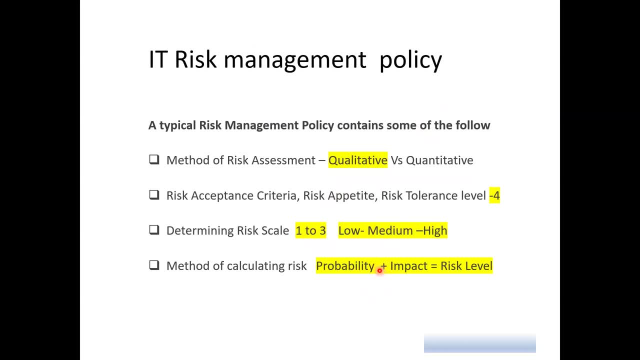 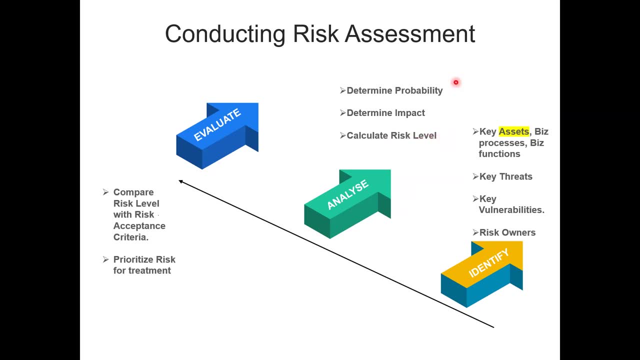 Remember we mentioned addition. that is our policy. So that means if we have adopted addition, it means that our risk level is now going to be four, Because we have one as probability, we have three as impact, So we add both of them together. 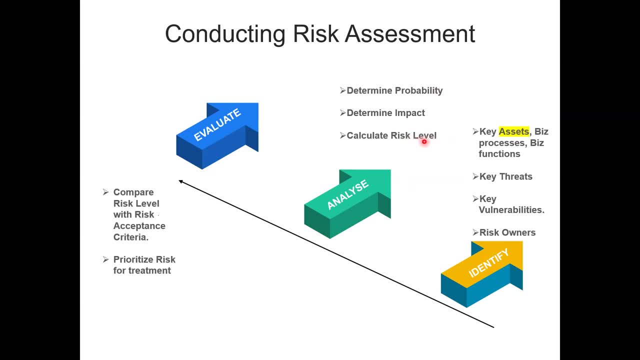 That is our risk level. And then you have not known your risk level for that particular Asset. And then what next will you do? You now look at comparing your risk level with the risk acceptance criteria. Now we have our risk level as four here. 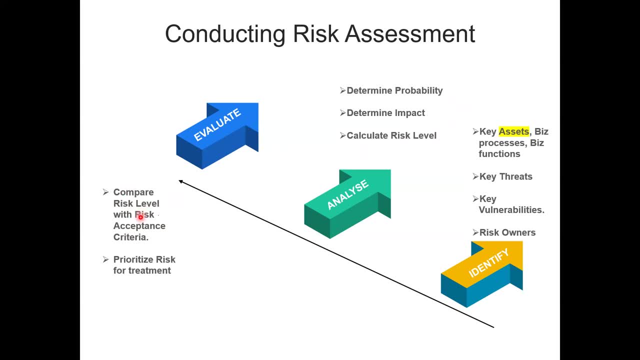 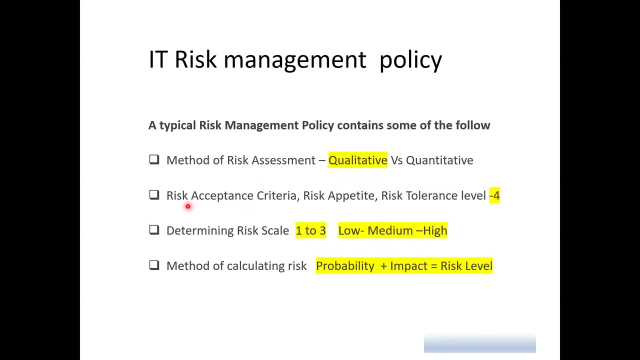 Let's go back to our policy. What does the policy say? What does it say about our risk acceptance level? And now the risk acceptance level. we go back to our policy. You say our risk. in our policy we say our risk acceptance level is four. 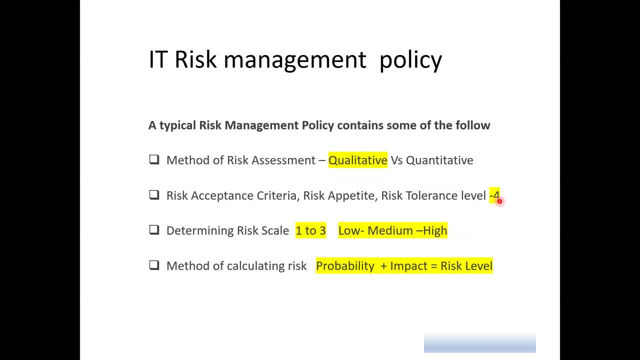 And what does that mean? That any risk that we calculate that is above four, it means we have to do something about it. So any risk that is between one or zero to four, that means we will accept it, We will do nothing about it. 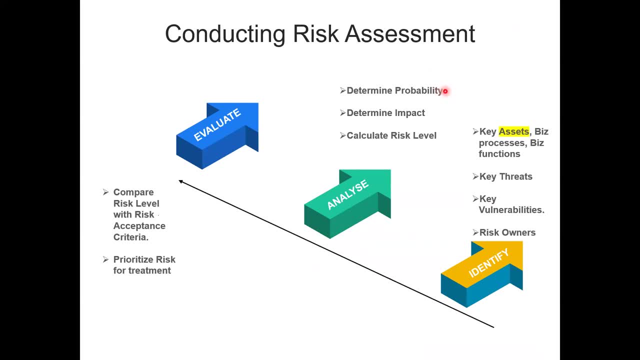 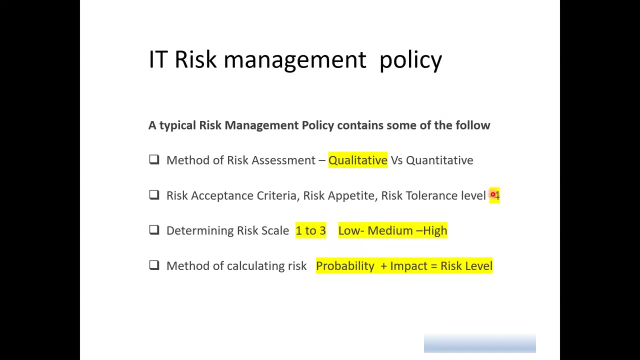 So if the risk we calculated here we have two and we have three, We have two as probability and we have three as impact- And our risk level becomes five, It means that our risk level is five, It means that it's above our risk acceptable level. 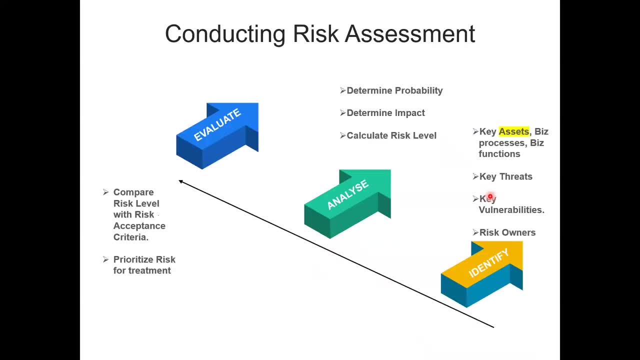 That means we have to do something about that risk. I hope you understand So now, having at the time you also you compare your risk level with your risk acceptance to determine whether you are going to accept the risk or treat the risk. And then the next thing is that you are going to now prioritize your risk for treatment. 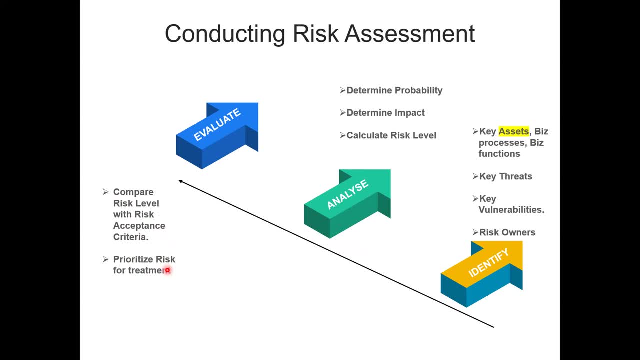 What does it mean? Remember that you are going to assess. You are going to conduct a risk assessment on different assets, not just one, Not just one. You are going to conduct a risk assessment on different assets, different processes. Then, at the end of the day, you are going to come up with risk level on many assets. 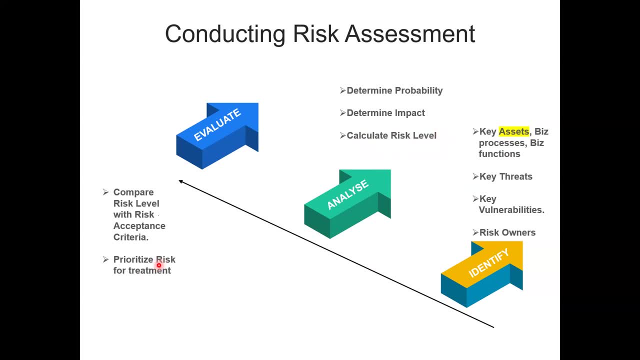 So some of them are going to be low, Some of them are going to be high, Some of them are going to be medium. So what it means that prioritizing your risk for treatment is that those risk levels are going to be high. So any risk that are above four level four, which is our maximum acceptable level risk. 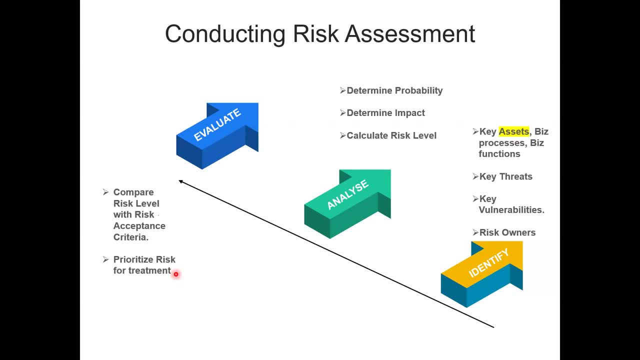 tolerance level, we are going to treat them. So any risk above that level it means that we are going to treat those risks. So we have to look at treating our risk based on their level of criticality. In other words, we are going to start from the highest rank risk. 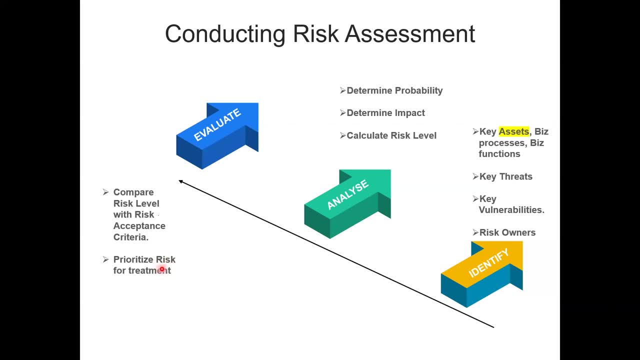 That is the most critical risk. We start treatment. We start treatment of risk from those critical ones when we come down to medium risks. So that is just a summary of how you conduct your risk assessment And then, briefly, we will just look at the next slide, which has to do with your risk treatment. 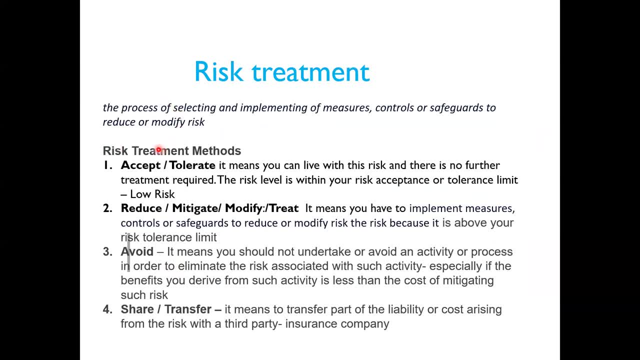 And then remember what is a risk treatment. Risk treatment is the process of selecting and implementing measures to control or measures to control the risk assessment. So you can use measures, controls or safeguards. The three words are used interchangeably. You can use measure, you can use control, you can use safeguard to reduce or modify your risk. 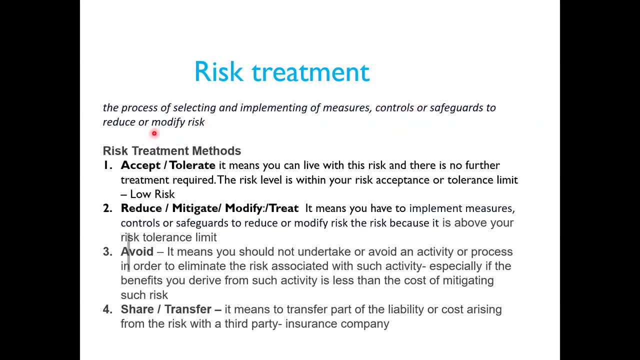 It can also be measures to treat, reduce or modify your risk. That means that if your risk level is above four, which is our tolerance limit, it means that we have to treat it or reduce it. If that, if risk level is four, that means we have to accept it. 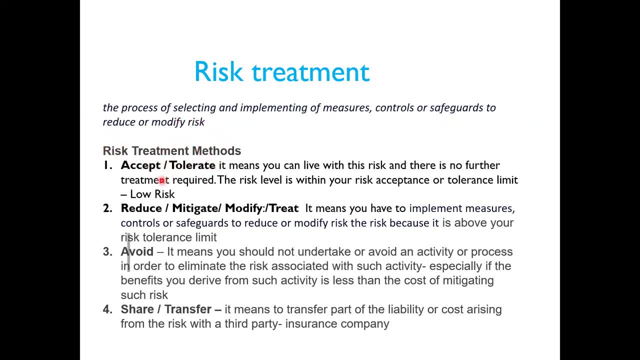 So there are four risk treatment options that we have Now. four of them, first of all, is accept. If it's accept, that means we can do. we do nothing about it. It is within our risk tolerance limit. No further action is required. 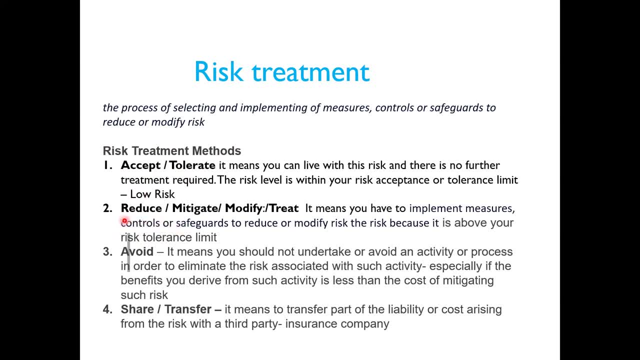 It's a low risk. And then the next option is to treat the risk People. you can say modify or mitigate, or reduce. These four terminologies are used interchangeably. It means that you have to implement controls. You have to implement controls, controls or safeguard. 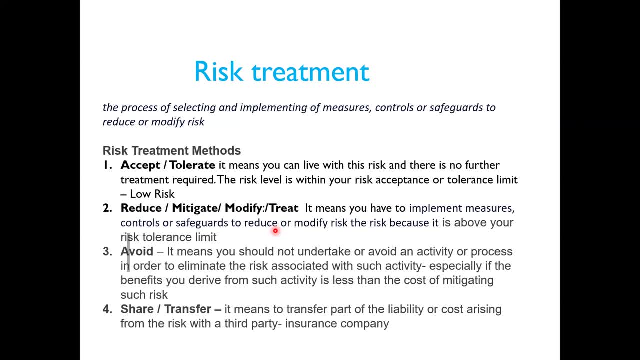 So, come on, somebody will say: where do you get these controls from? Controls are most times are in your standard. If you are using ISO 27001,, for example, your controls are your NSA. If you are using NIST, your controls are there in the NIST framework. 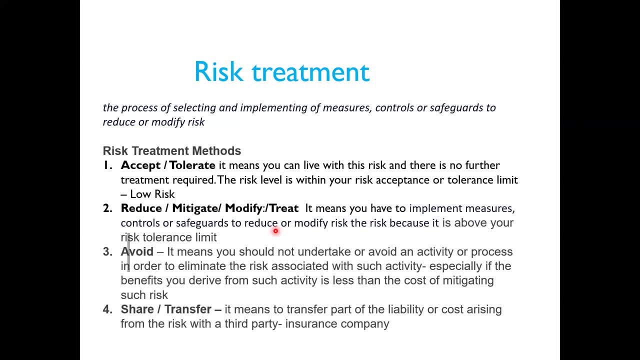 So the controls- I mean the measures or safeguards you want to use to ensure that the risk does not happen. Or, if it does happen, how can you bring the risk down to an acceptable level. So when you treat your risk, after treating your risk, it is no longer a high risk because you have put controls in place. 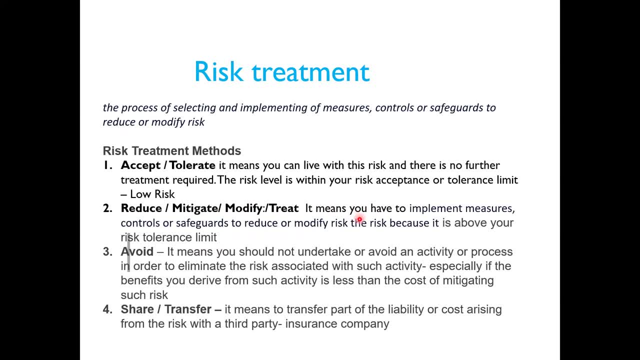 For example, if for any reason, You park your car outside and you didn't lock it, thieves come and take away and steal your property. You have suffered a risk. steal your car. you have suffered a risk. or steal something inside your car. 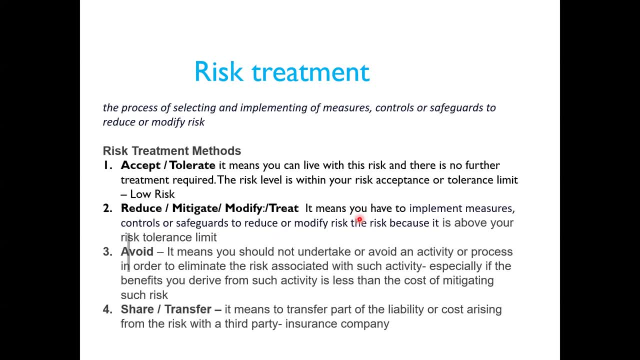 Maybe take something valuable inside the car. You have suffered a loss. that's a risk. So what are you going to do next? You are going to implement controls to ensure that you do not suffer such a risk again by actually locking your car. 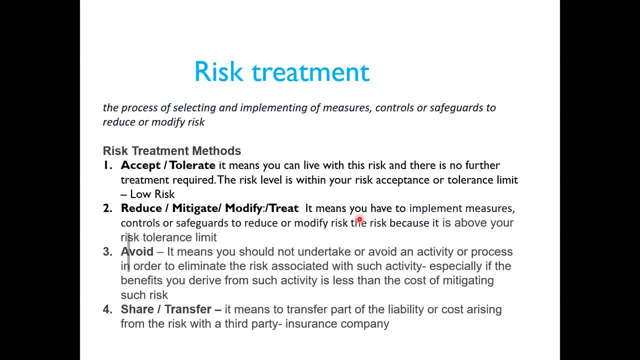 And that is it. Control, that is a measure. You have deployed a control to mitigate that risk. So what you have done, if you haven't deployed the control to mitigate that risk, your risk will now return to acceptable level because it has been treated. 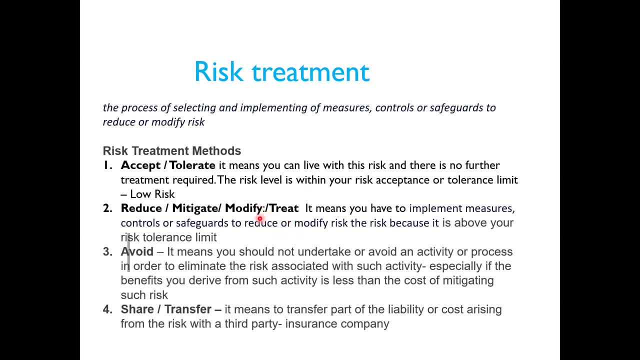 Mostly, yeah, so mostly. mostly- after treating your risk ideally, it becomes a residual risk. You know, residual risk is a risk that you know. after I mean implementing the controls or the measure, your risk becomes, the risk becomes a residual risk after the risk has been treated. 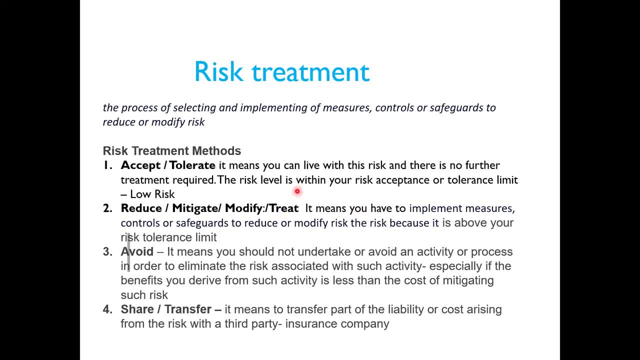 So the idea of treating risk is to make sure that you bring the risk back to an acceptable level. Other ways of treating risk is to avoid doing something or taking an activity or a process in order to eliminate the risk associated with that activity. For example, if your company 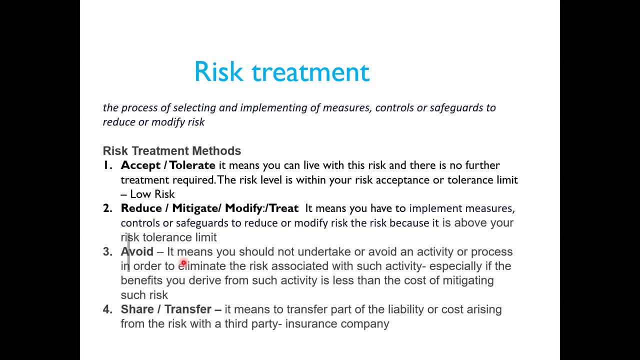 If your company, If your company implement work from home and people use- I mean sorry, not work from home, Let me say yeah, work from home and people bring, use their own device to connect to your network. You can, you can. 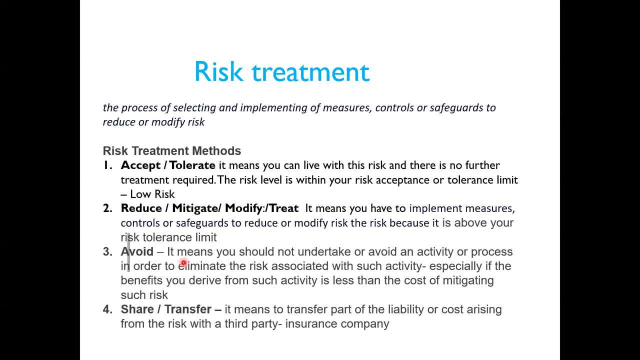 And the device. people use their personal devices, like personal phones, rather than company phones, to connect to your company network. What do you do If the if that is causing the company too much risk or too much problem? so what you can do is to stop using, stop people from connecting to your network. 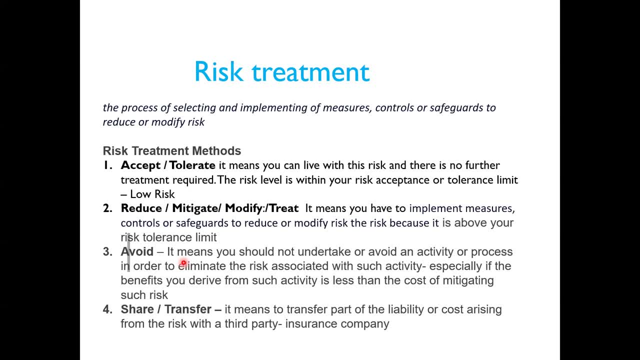 Okay, Okay, Okay. So if you're using their personal device, you have to restrict them from connecting. restrict them to connecting to your network only with company devices. So what have you done? You have decided to avoid that process. You have avoided using personal devices. 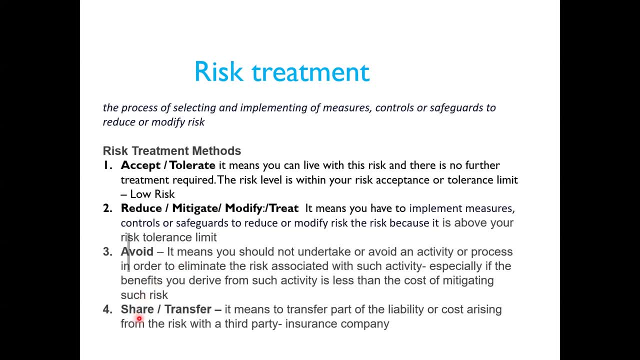 So that is what we mean by risk avoidance. So another option is to share transfer. So any risk you have you want to treat, so you have an option to transfer Partly, Partly So you can take part of the risk to insurance company by taking an insurance, cyber insurance, liability insurance, cyber liability insurance. 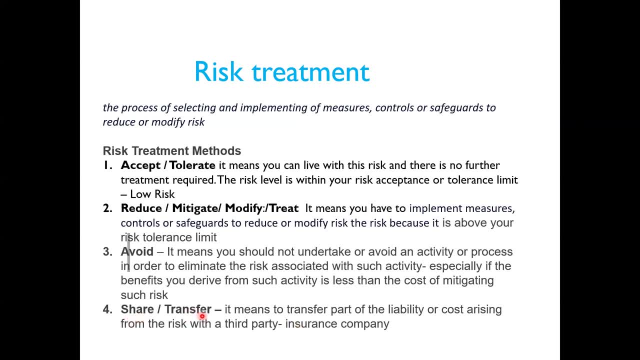 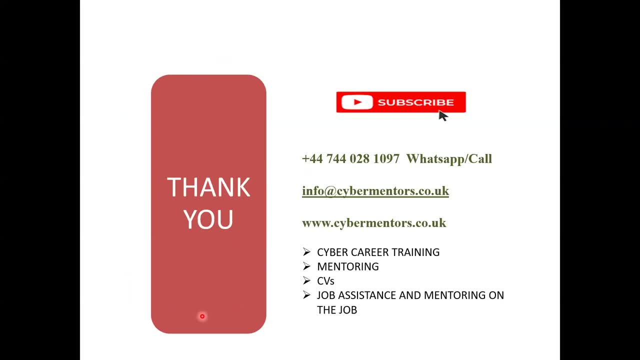 So that is what you mean by transferring or sharing the risk, And I hope you enjoyed this video. If you did, please don't forget, like I said, to subscribe. subscribe to this video. These are our contact details. um our services include the cyber training, mentoring, cv, cv preparation and review also. 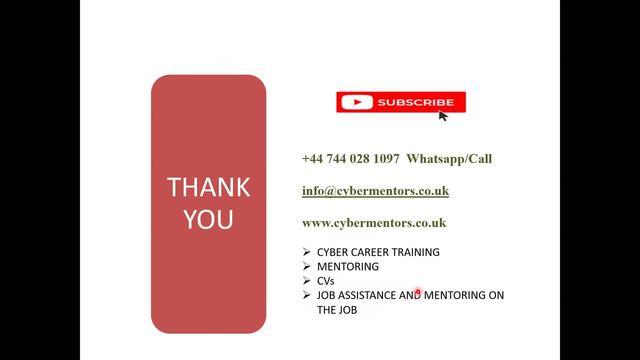 help with job assistance and then um mentoring you when you get your job. so that's a summary of our services. you can check out our website for more details on of our services in terms of mentoring and training. so don't forget to subscribe to our video. thank you very much and stay blessed.